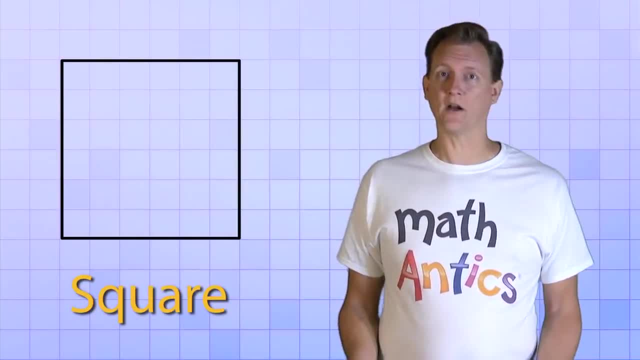 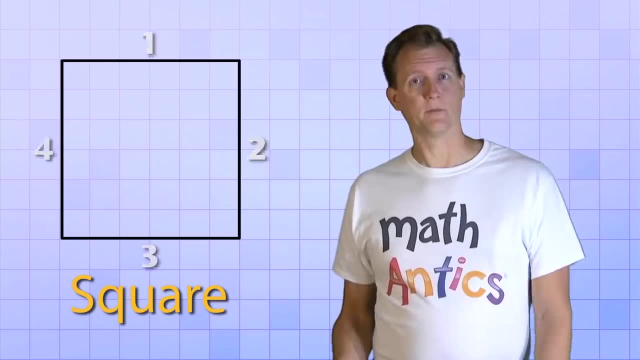 You should recognize this shape. of course It's a square, And a square is a special kind of quadrilateral. It's a quadrilateral because it has four sides, And it's special because all four of those sides are exactly the same length. 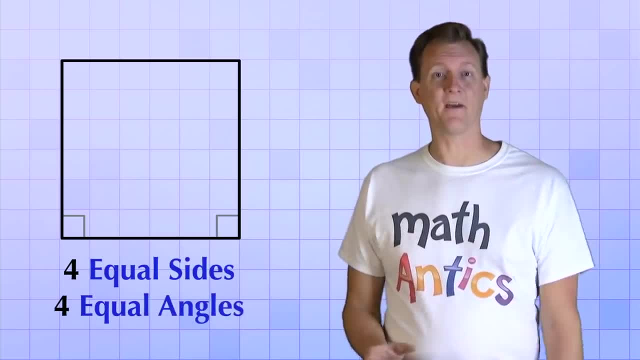 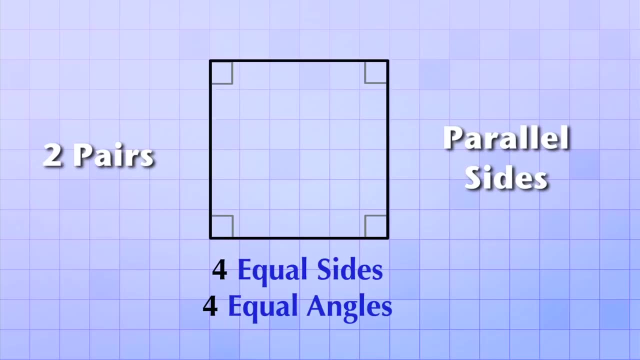 And all four of its angles are exactly the same size. In fact, they're all right angles. Notice also that a square is formed by two pairs of parallel sides. These two opposite sides are parallel and these two opposite sides are parallel. We'll see why that's important in a few minutes. 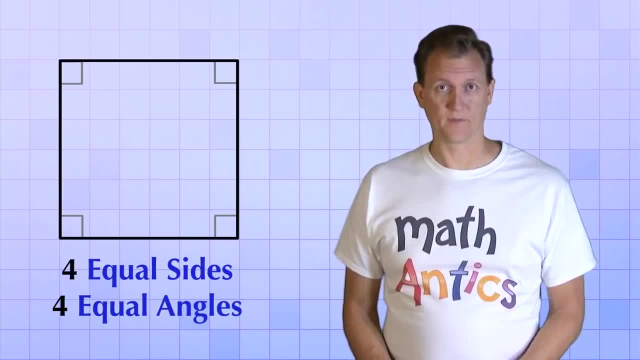 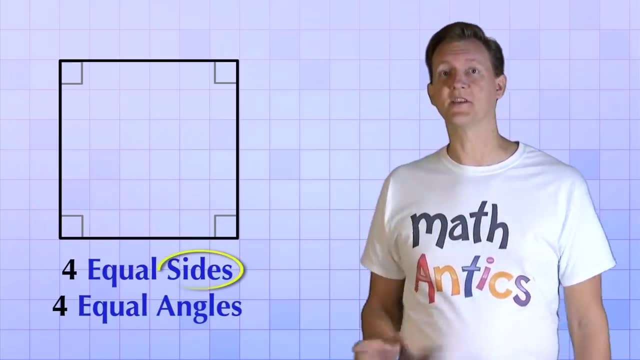 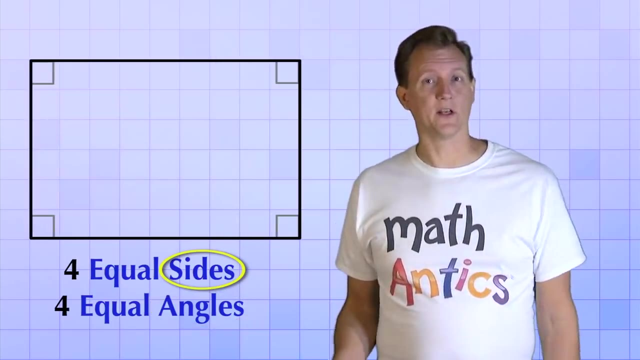 Okay, so squares are an important type of quadrilateral, But we're going to make some changes to the square to see what other types of quadrilaterals there are. The two things that we can change are the sides and the angles. Let's start by changing the sides. Let's stretch our square in one direction. 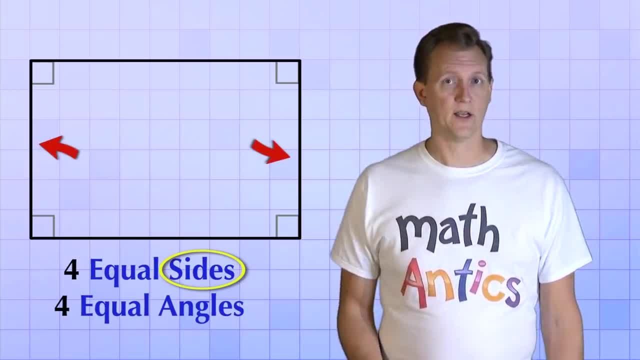 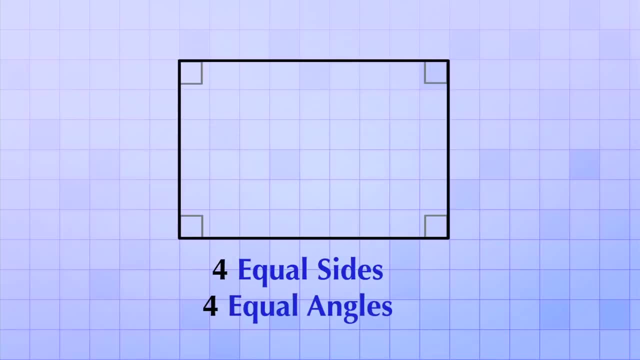 so that one pair of sides is now longer than the other pair. This is what we call a rectangle. A rectangle is a quadrilateral that still has four equal angles. Notice that when we stretch the square, the angles didn't change at all. 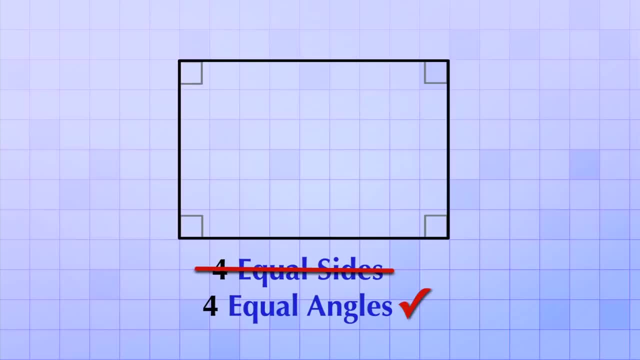 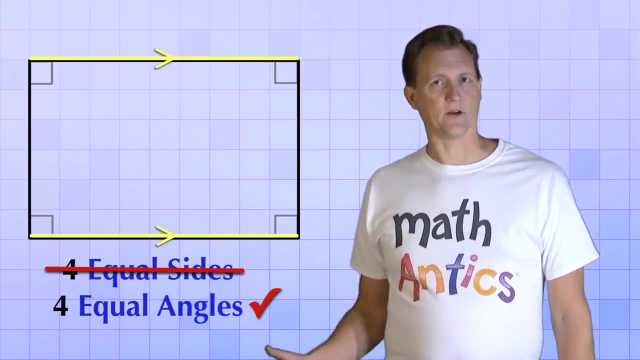 It does NOT have four equal sides. Again, notice that, just like a square, a rectangle is made from two pairs of parallel sides. Alright, so that's a rectangle. But going back to our square, what if, instead of changing the sides, we had just changed the angles? 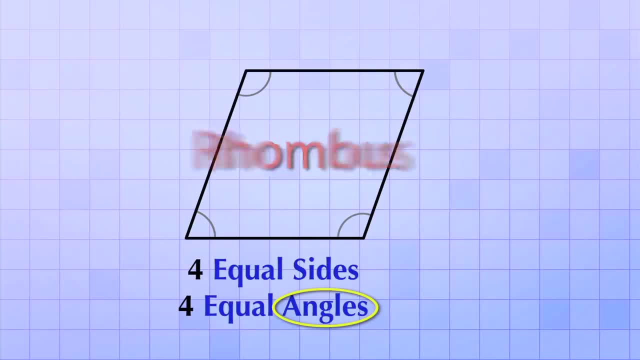 Like this: Ah, What we have now is called a rhombus. A rhombus is a quadrilateral that still has four equal sides, but it does not have four equal angles, And, once again, square and rectangle. the rhombus is made from two pairs of parallel sides. 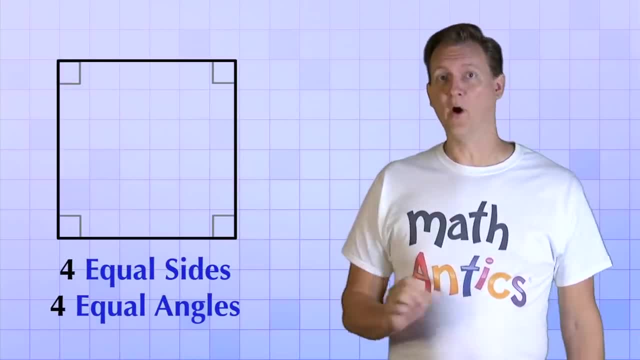 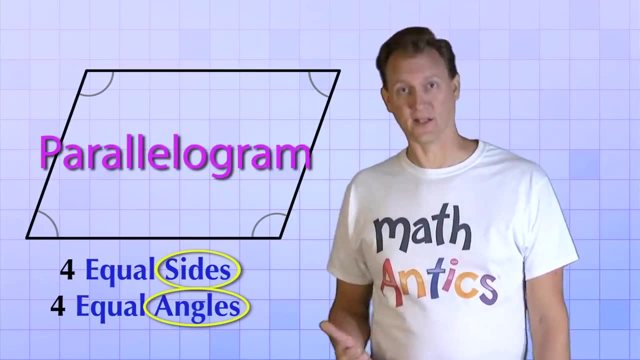 Okay, going back once more to our square, what if we try changing both the sides and the angles? Here's what we end up with and we call it a parallelogram. It's called a parallelogram because, even though its sides are not all equal. 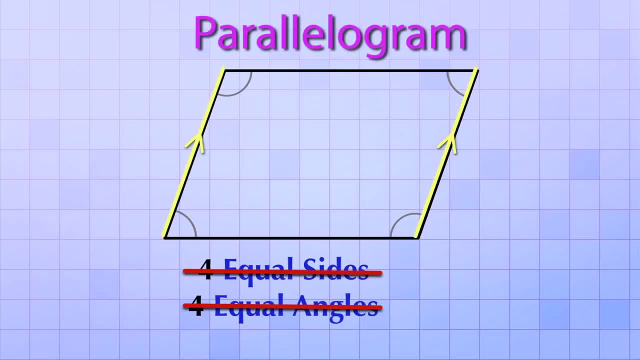 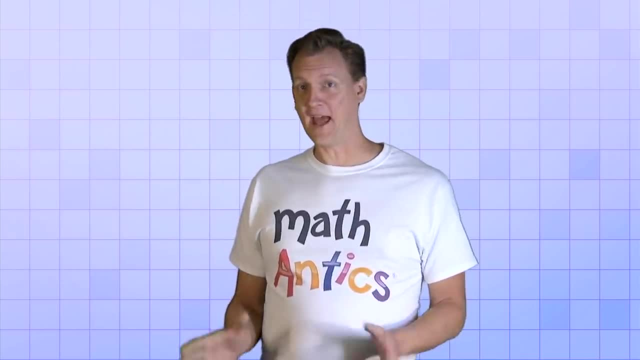 and its angles are not all equal, it's still made from two pairs of parallel sides. Get it Parallel Parallelogram. Now wait a second. if that's the definition of a parallelogram, a quadrilateral that's made from two pairs of parallel sides. 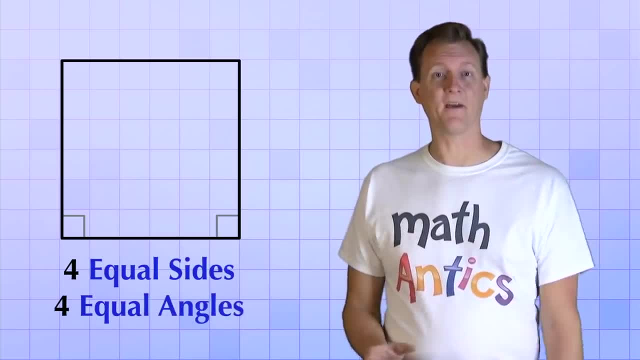 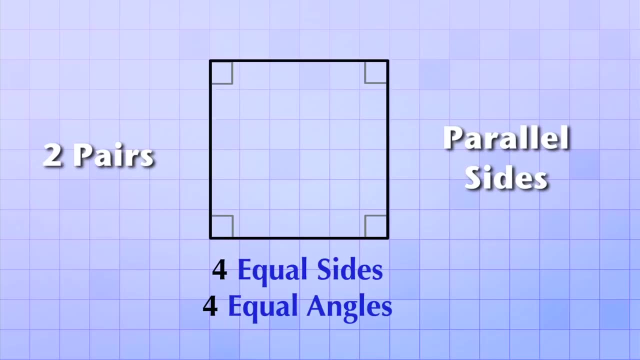 And all four of its angles are exactly the same size. In fact, they're all right angles. Notice also that a square is formed by two pairs of parallel sides. These two opposite sides are parallel and these two opposite sides are parallel. We'll see why that's important in a few minutes. 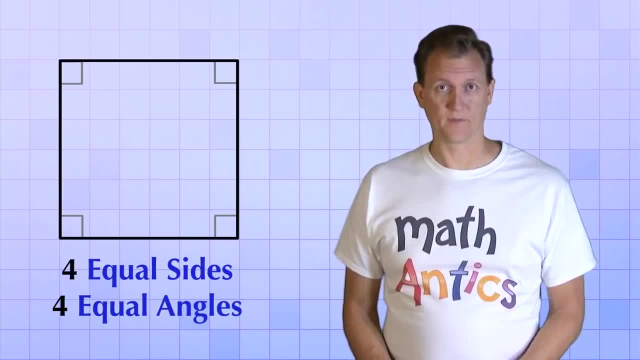 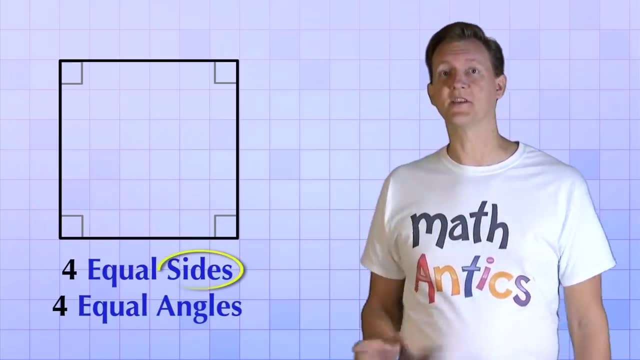 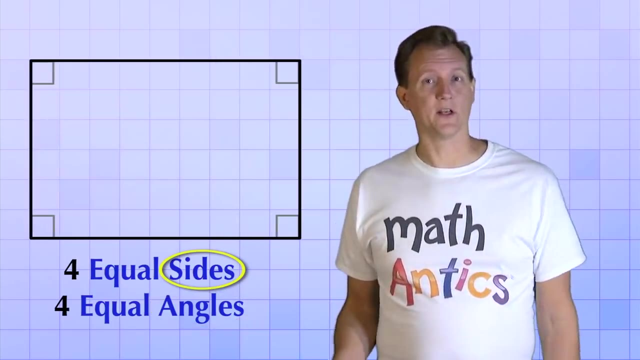 Okay, so squares are an important type of quadrilateral, But we're going to make some changes to the square to see what other types of quadrilaterals there are. The two things that we can change are the sides and the angles. Let's start by changing the sides. Let's stretch our square in one direction. 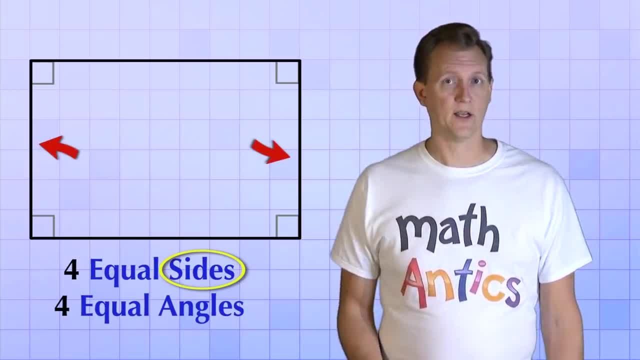 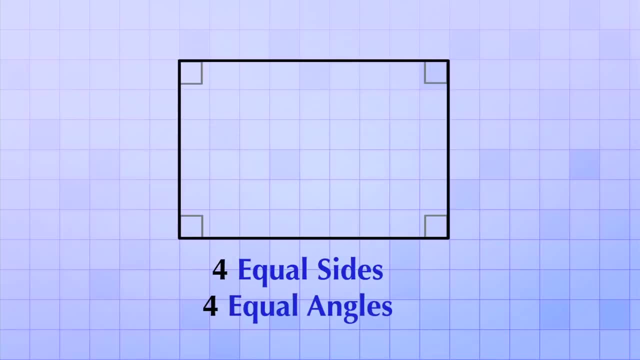 so that one pair of sides is now longer than the other pair. This is what we call a rectangle. A rectangle is a quadrilateral that still has four equal angles. Notice that when we stretch the square, the angles didn't change at all. 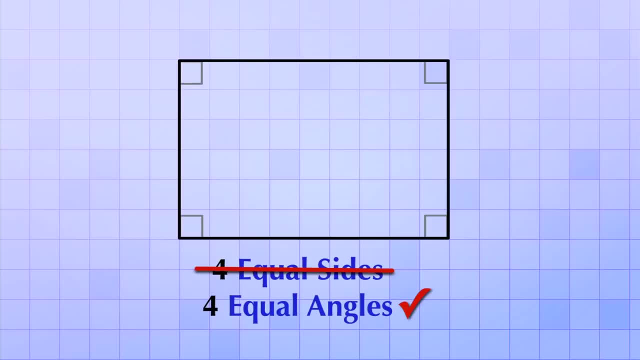 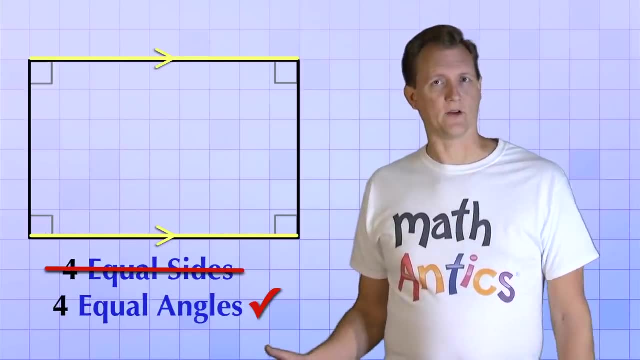 It does not have four equal sides. Again, notice that, just like a square, a rectangle is made from two pairs of parallel sides. Alright, so that's a rectangle. But going back to our square, what if, instead of changing the sides, 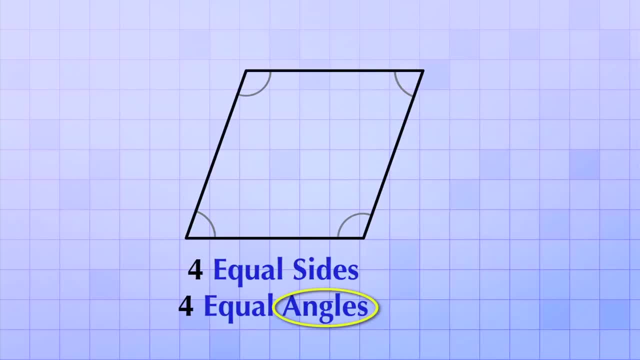 we had just changed the angles like this. Ah, what we have now is called a rhombus. A rhombus is a quadrilateral that still has four equal sides, but it does not have four equal angles And, once again, just like the square, it's made from two pairs of parallel sides. 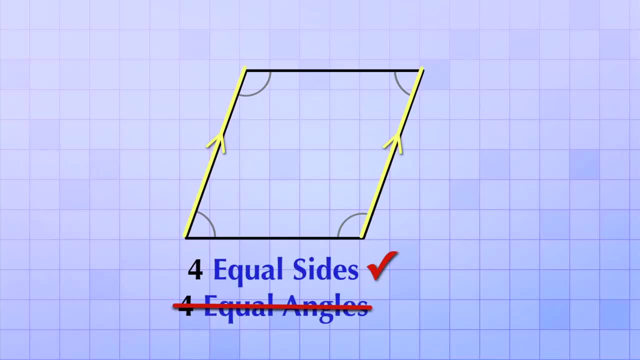 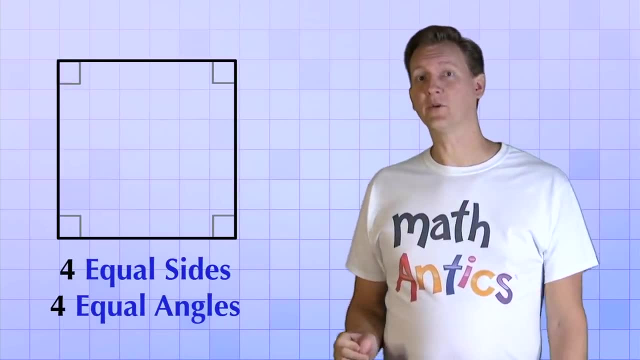 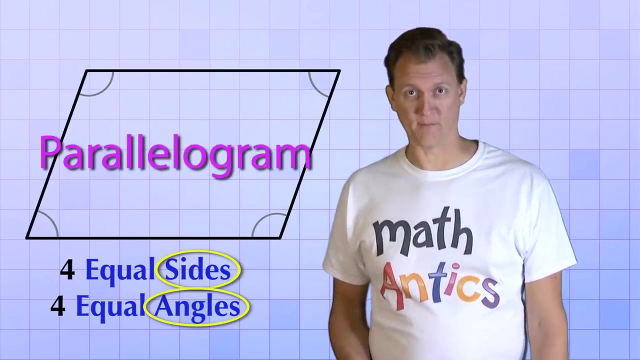 Just like the square and rectangle, the rhombus is made from two pairs of parallel sides. Okay, going back once more to our square, What if we try changing both the sides and the angles? Here's what we end up with, And we call it a parallelogram. 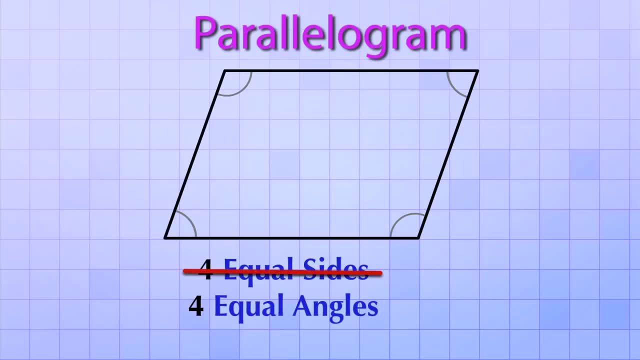 It's called a parallelogram because, even though its sides are not all equal and its angles are not all equal, it's still made from two pairs of parallel sides. Get it Parallel Parallelogram. Now wait a second. If that's the definition of a parallelogram. 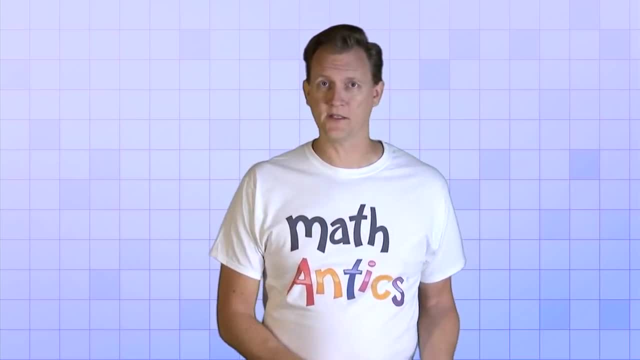 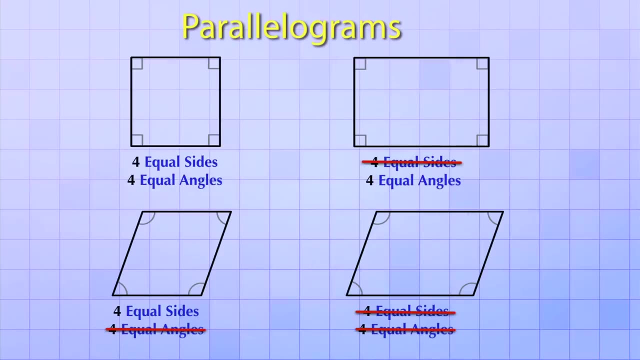 a quadrilateral that's made from two pairs parallel sides, then wouldn't all of these other shapes be parallelograms too? Exactly, All of these shapes are parallelograms, just like they're all quadrilaterals. It's just that we have special names for them if their angles are all equal. 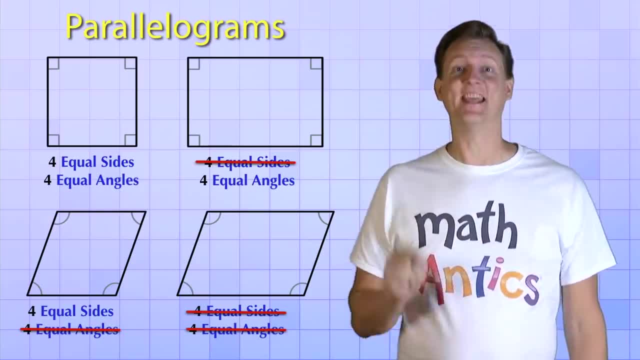 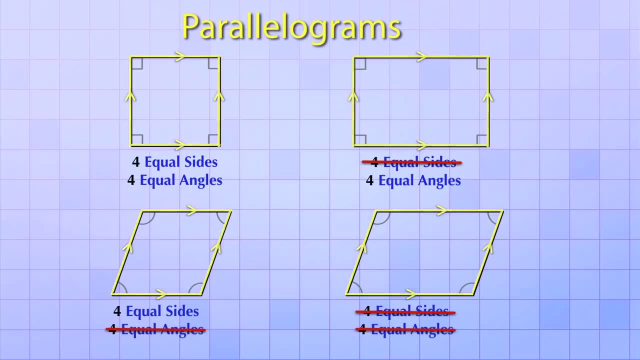 then wouldn't all these other shapes be parallelograms too? Exactly, All of these shapes are parallelograms, just like they're all quadrilaterals. It's just that we have special names for them if their angles are all equal or if their sides are all equal. 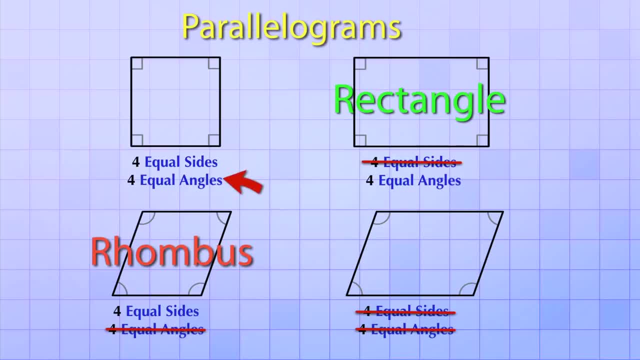 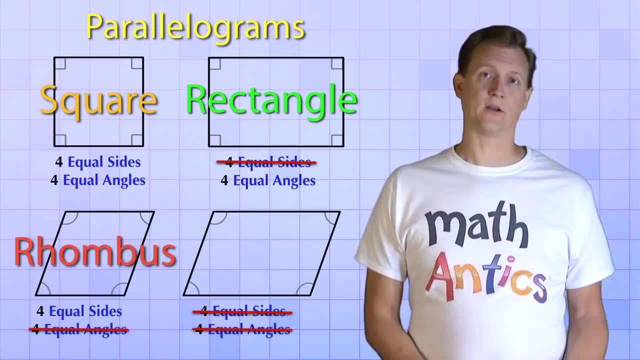 or if both their sides and their angles are all equal. Okay then, if all the quadrilaterals we've seen so far are examples of parallelograms, what's an example that's not a parallelogram? Well, to see one. let's start over with our square again. 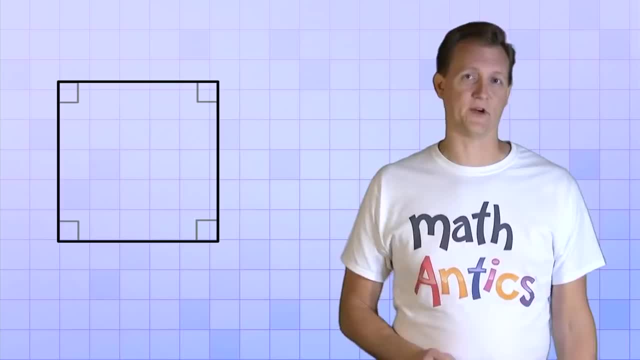 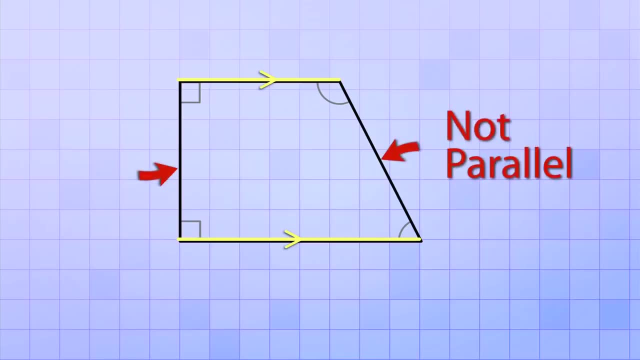 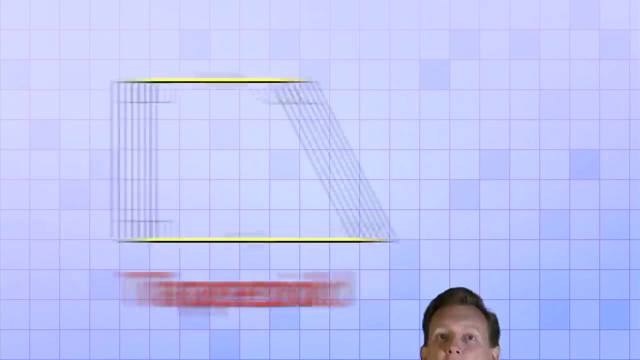 but this time we're going to change it by moving just one of its vertices, like so: Now one of the pairs of sides is still parallel, but the other is not, and a quadrilateral that has only one pair of parallel sides is called a trapezoid. 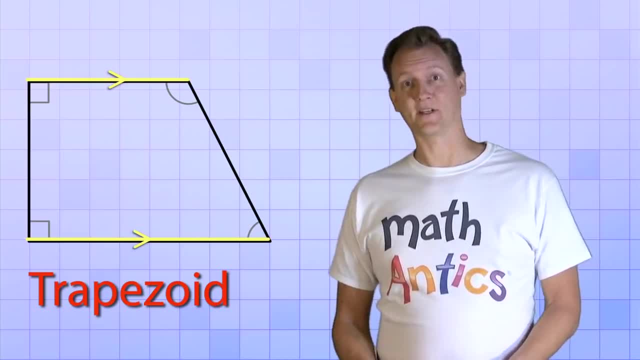 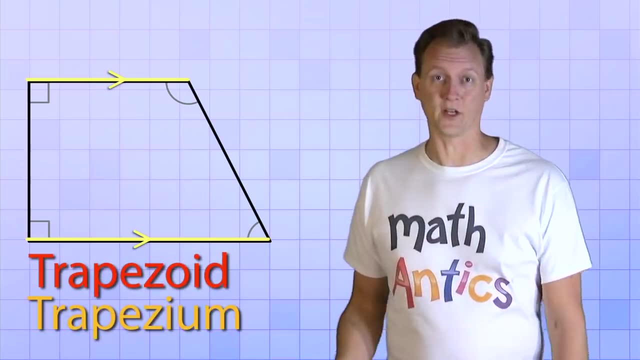 Well, actually this is where classifying quadrilaterals gets a little messy, And that's because this sort of shape is called a trapezoid in America, but it's called a trapezium in other countries like the UK. 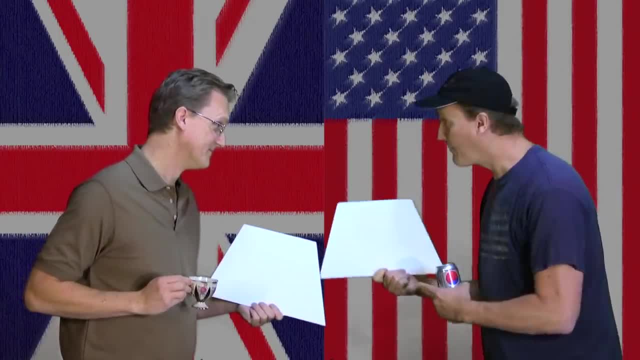 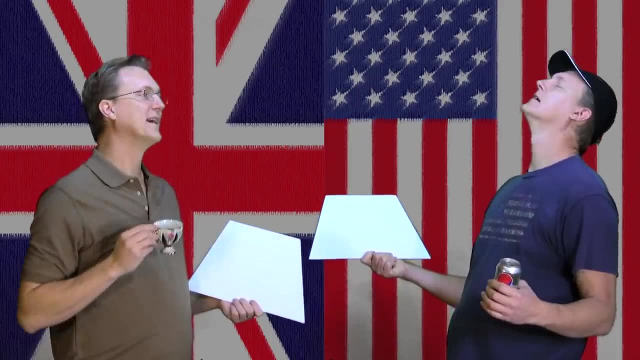 Trapezoid Trapezium. Trapezoid Trapezium, It's a trapezoid. Ahh, At least you actually need that. gotta make it to Michigan. At least they both start with the word TRAP, so it's not too confusing… yet 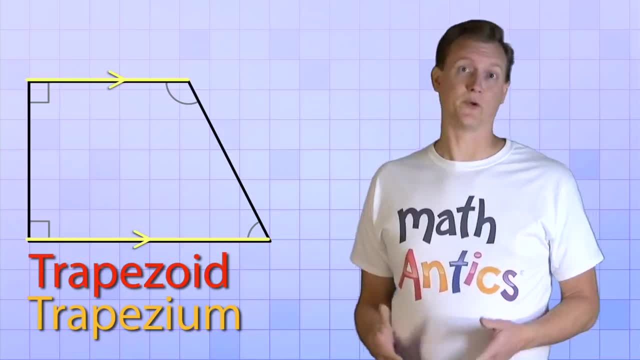 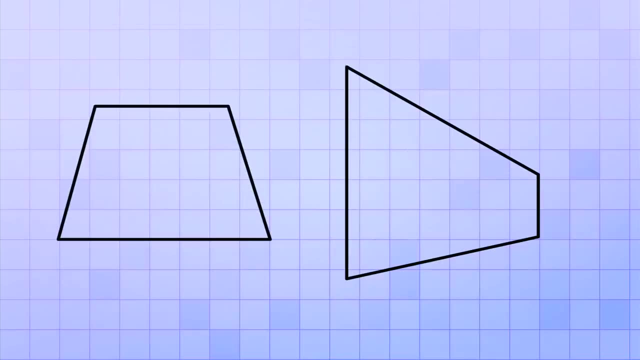 Okay, so this quadrilateral is a trapezoid or trapezium, because it has only one pair of parallel sides and the other sides are not parallel. Here are a couple more examples of quadrilaterals that have only one set of parallel sides. 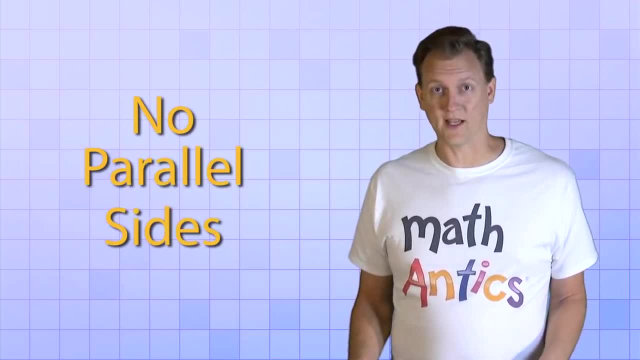 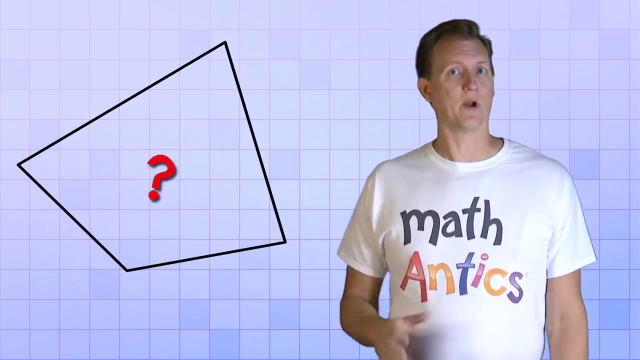 Alright, then what about quadrilaterals that have no parallel sides at all, like this one? These opposite sides are not parallel, and these opposite sides aren't parallel either. So what do we call this kind of polygon? Ah, now here's the really confusing part. 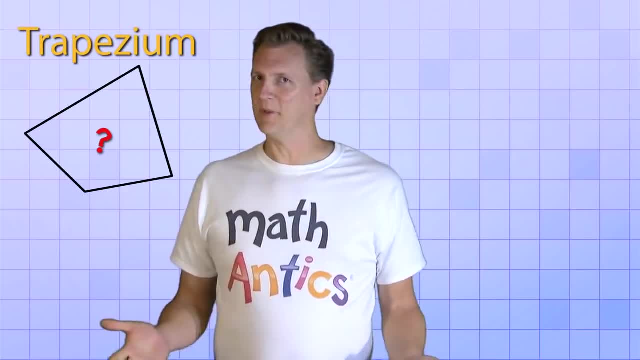 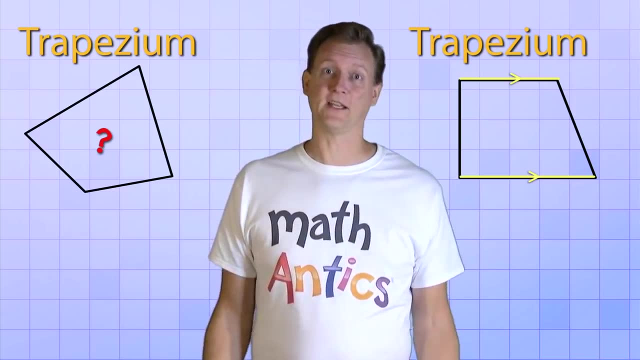 In America this is sometimes called a trapezium, But isn't that what they call a quadrilateral with only one pair of parallel sides in the UK? Yup, Unfortunately, the same word is used to describe two different things in two different countries. 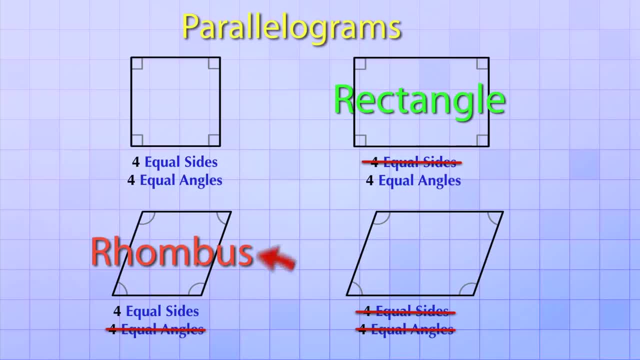 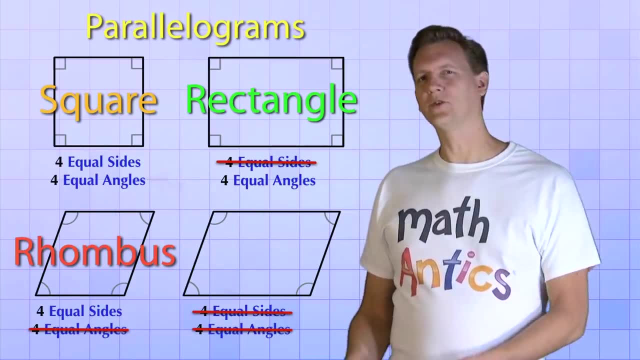 or if their sides are all equal, or if both their sides and their angles are all equal- a square. OK, then if all the quadrilaterals we've seen so far are examples of parallelograms, what's an example that's NOT a parallelogram? 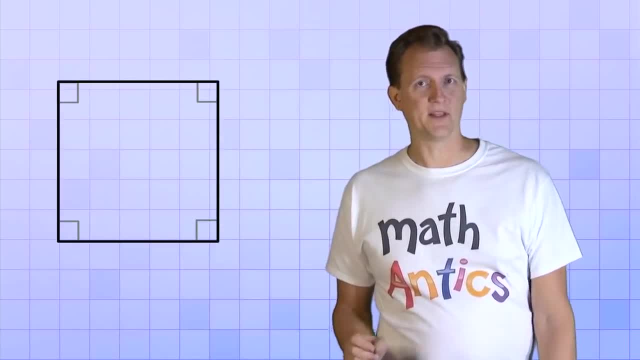 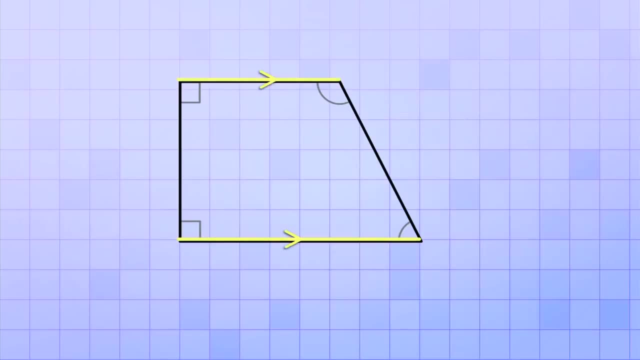 Well, to see one. let's start over with our square again, but this time we're going to change it by moving just one of its vertices, like: so: Now one of the pairs of sides is still parallel, but the other is not. 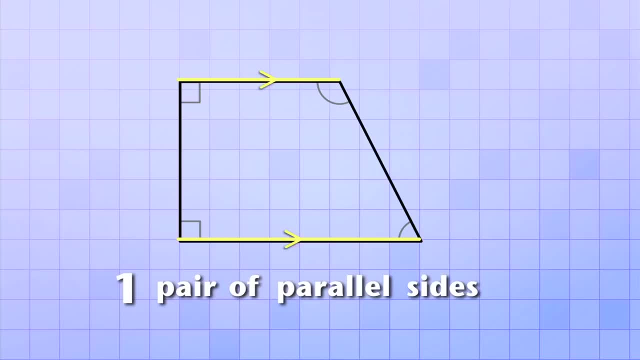 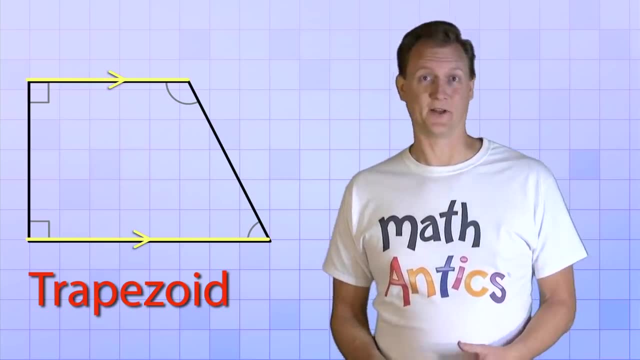 and a quadrilateral that has only one pair of parallel sides is called a trapezoid. Well, actually this is where classifying quadrilaterals gets a little messy, and that's because this sort of shape is called a trapezoid in America. 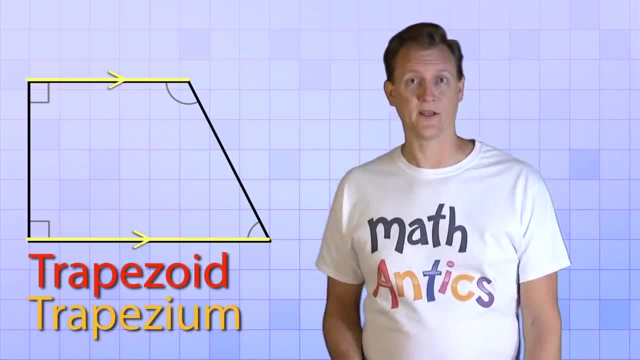 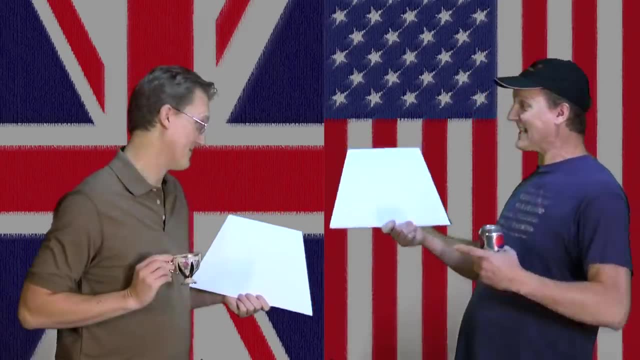 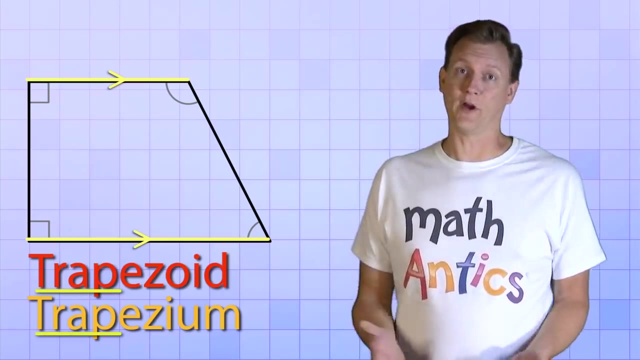 but it's called a trapezium in other countries like the UK: Trapezoid Trapezium, Trapezoid Trapezium, It's a trapezoid Ugh. At least they both start with the word trap, so it's not TOO confusing… yet 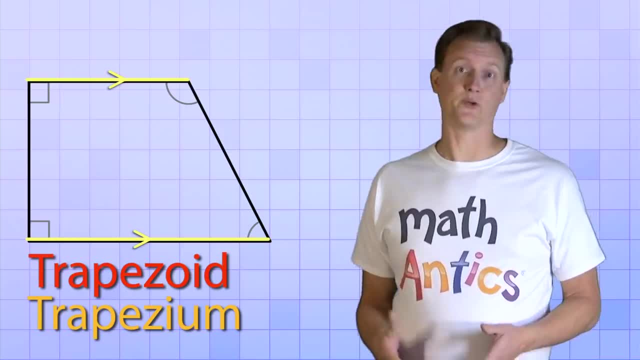 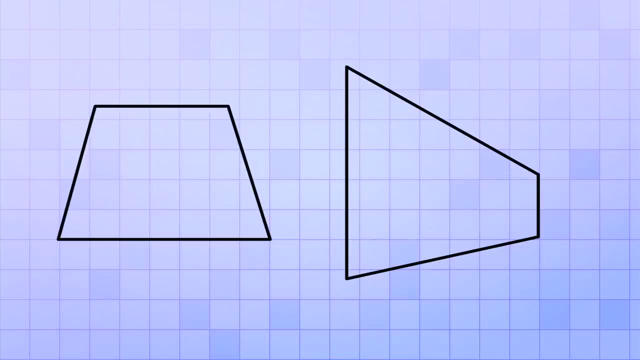 OK, so this quadrilateral is a trapezoid or trapezium because it has only one pair of parallel sides and the other sides are not parallel. Here are a couple more examples of quadrilaterals that have only one set of parallel sides. 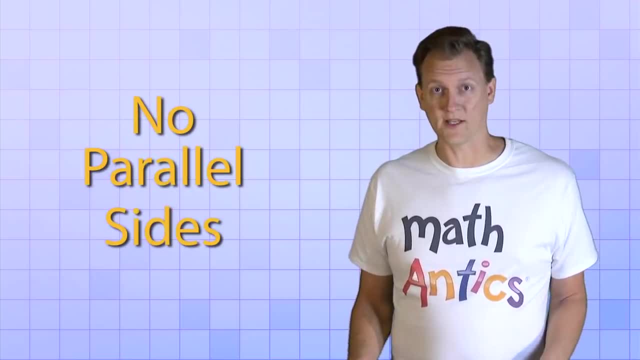 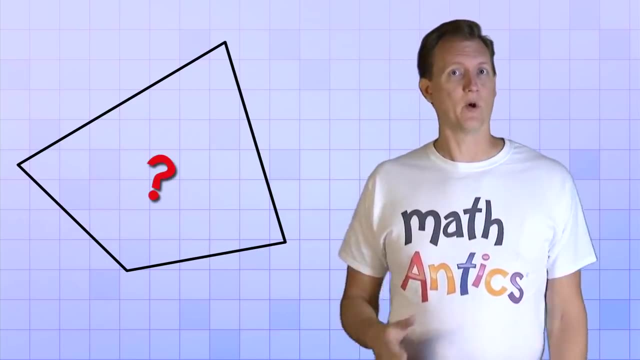 Alright, then what about quadrilaterals that have no parallel sides at all, like this one? These opposite sides are not parallel, and these opposite sides aren't parallel either. So what do we call this kind of polygon? Ah, now here's the really confusing part. 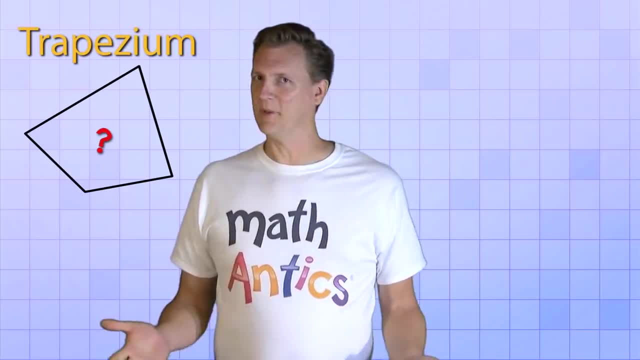 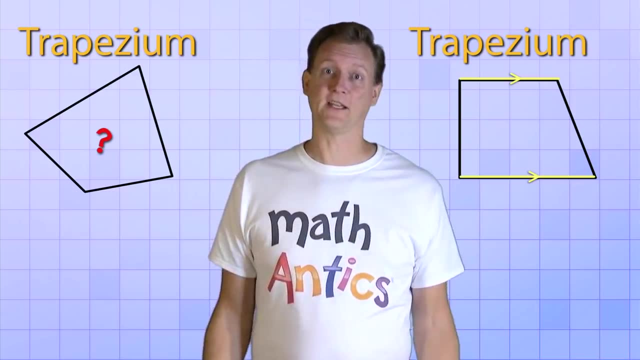 In America this is sometimes called a trapezium, But isn't that what they call a quadrilateral with only one pair of parallel sides in the UK? Yep, Unfortunately, the same word is used to describe two different things in two different countries. 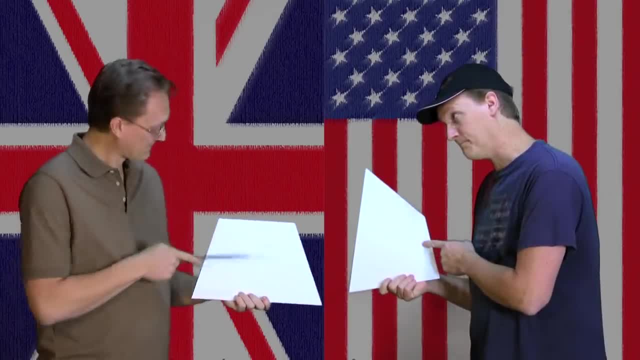 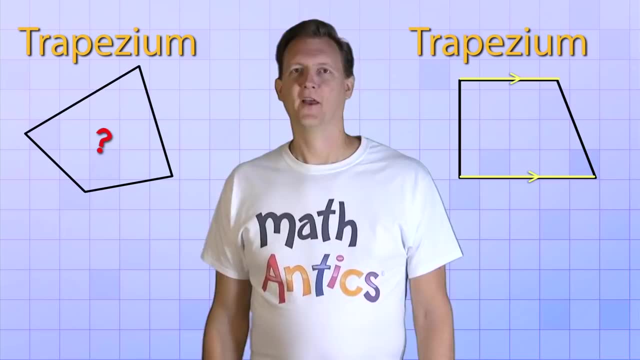 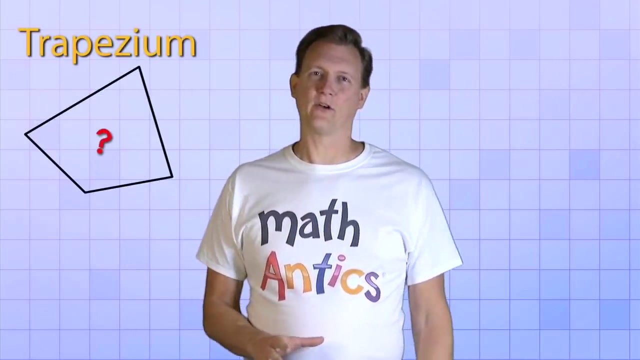 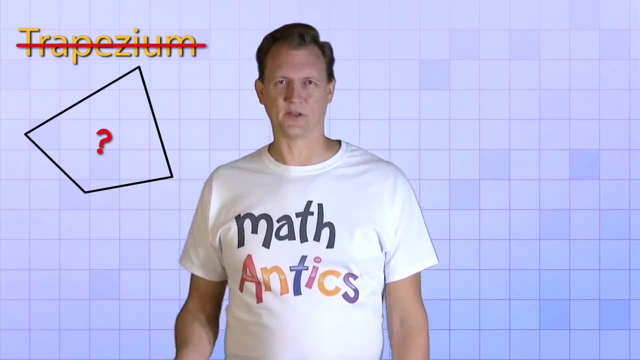 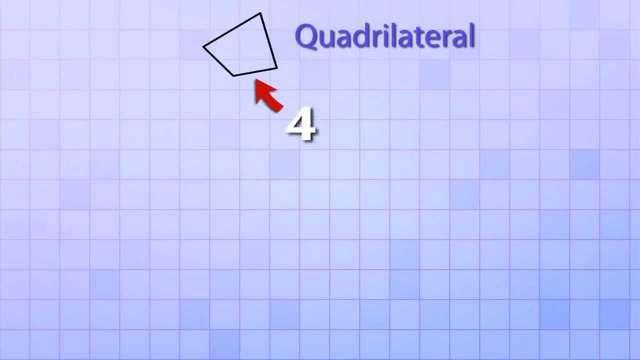 no parallel sides, a trapezium. We don't think it needs a special name, so we're just going to call it a quadrilateral. So to summarize: any polygon that has exactly four sides is called a quadrilateral, And if it has no parallel sides, 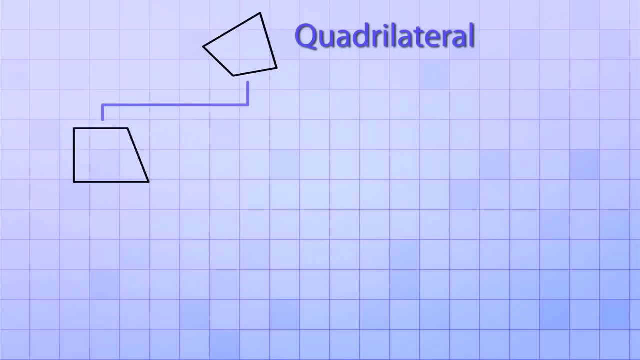 we'll just call it a quadrilateral. But if it has one and only one pair of parallel sides, we call it a trapezoid or a trapezium, Or if it has two pairs of parallel sides, we call it a parallelogram. 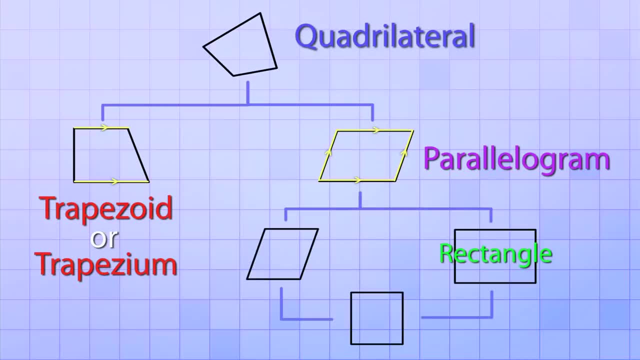 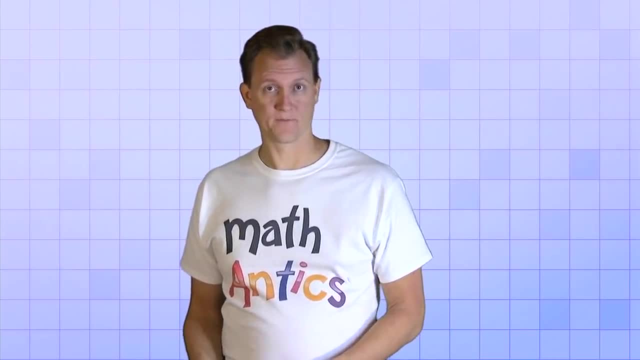 And you've already seen that there's several types of parallelograms called rectangles, rhombuses and squares. Alright, so that's the basics of classifying quadrilaterals, And there's a few other special types of quadrilaterals. 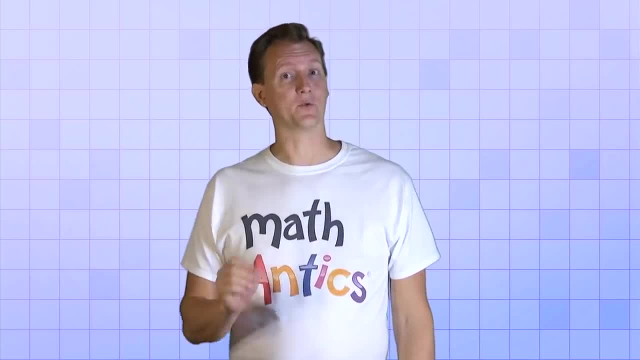 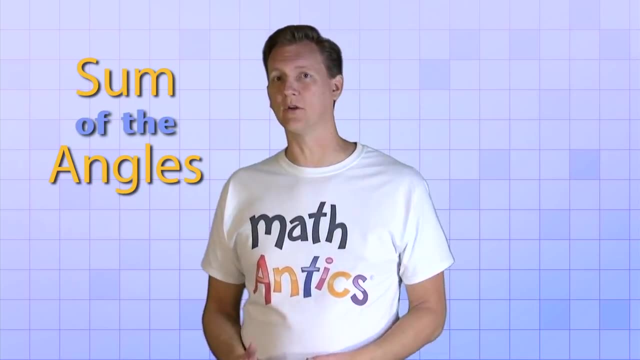 but we've learned the most important ones. But there is one more really important thing you need to know about quadrilaterals. You need to know that the sum of the angles of a quadrilateral is always 360 degrees. Now, that's pretty obvious for a square or a rectangle. 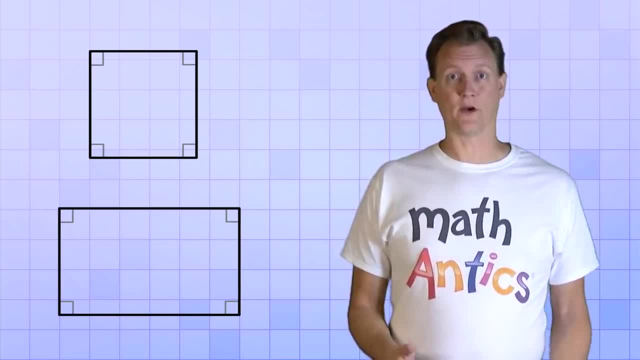 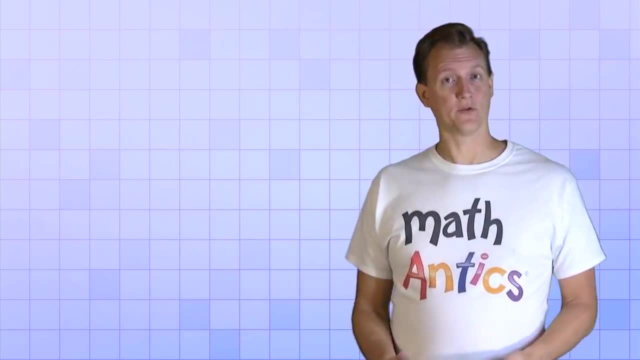 Those shapes have four right angles And since we know that a right angle is 90 degrees, 4 times 90 gives us 360.. But to see that it's also true for any quadrilateral, let's have a look at these four angles. 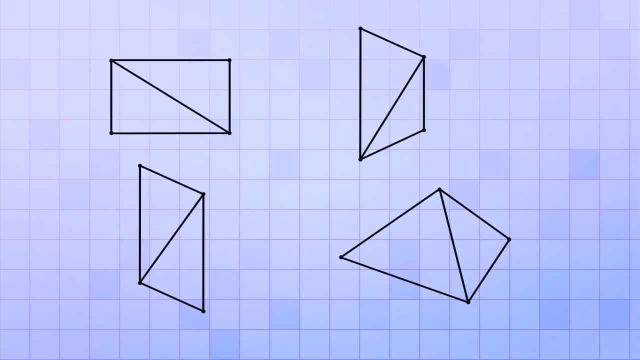 We've already heard different examples. Watch what happens when we draw a line on each of them. between a pair of opposite vertices, Each of the quadrilaterals got divided into two triangles. In the triangles video, we learned that the sum of the angles of a triangle is always 180 degrees. 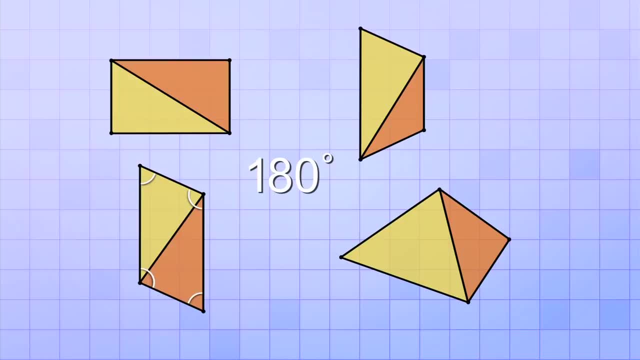 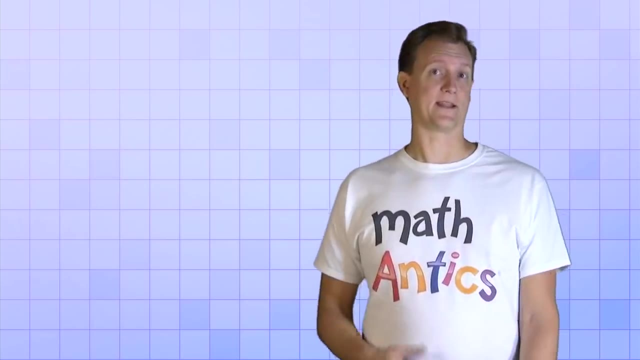 So it's not too hard to see that, since the angles of a quadrilateral form two triangles, the sum of those angles would be 2 times 180 degrees, which is 360.. Knowing that the angles of a quadrilateral add up to 360 degrees can help you solve problems like this one. 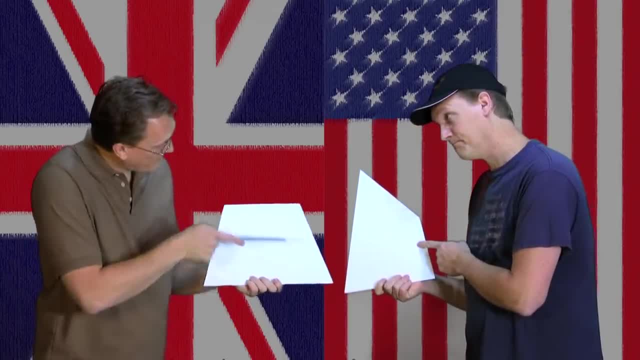 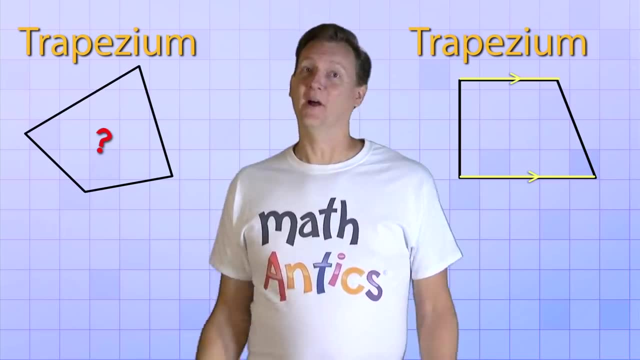 TRAPEZIUM, TRAPEZIUM, TRAPEZIUM, TRAPEZIUM, TRAPEZIUM, TRAPEZIUM. Well, at least they both like football. But to keep things clear, at Math Antics we're not going to call a quadrilateral that has. 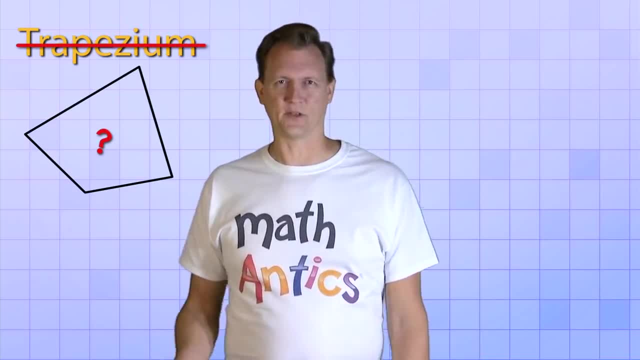 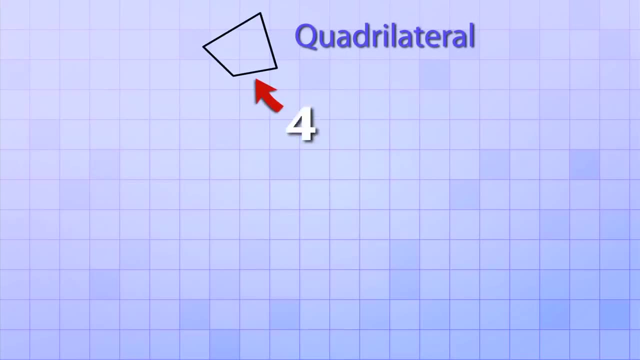 no parallel sides, a trapezium. We don't think it needs a special name, so we're just going to call it a quadrilateral. So to summarize: any polygon that has exactly four sides is called a quadrilateral, And if it has no parallel sides, 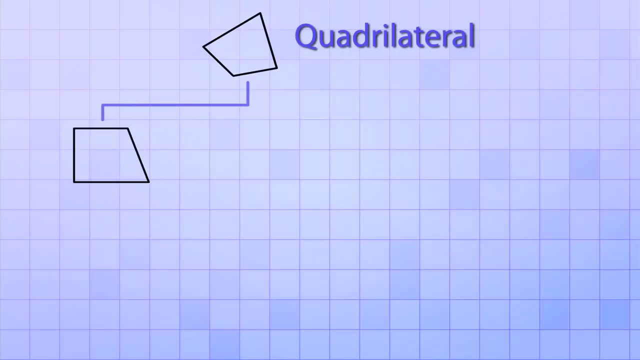 we still just call it a quadrilateral. But if it has one and only one pair of parallel sides, we call it a trapezoid or a trapezium, Or if it has two pairs of parallel sides, we call it a parallelogram. 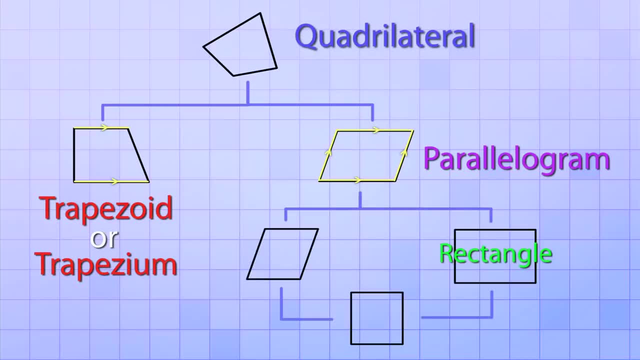 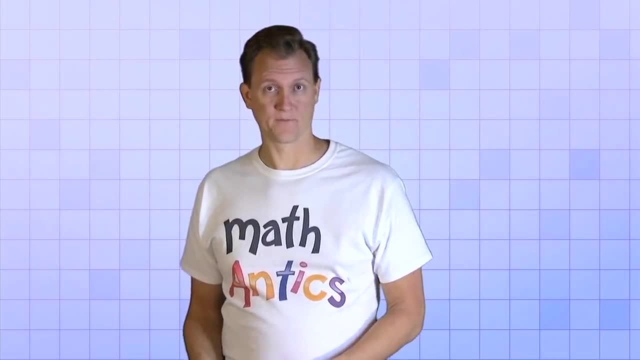 And you've already seen that there's several types of parallelograms called rectangles, rhombuses and squares. Alright, so that's the basics of classifying quadrilaterals, And there's a few other special types of quadrilaterals, but we've learned the most important one. 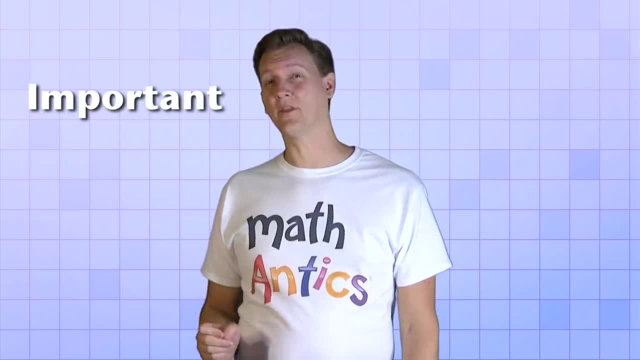 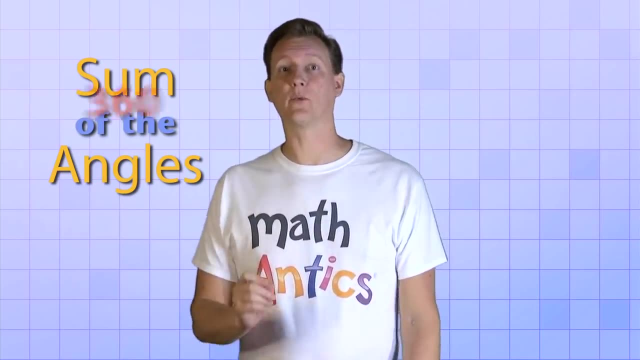 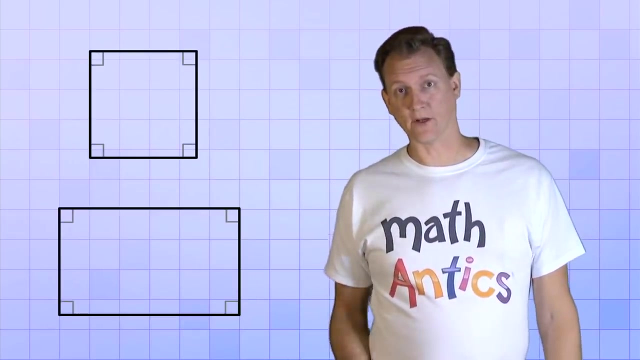 But there is one more really important thing you need to know about quadrilaterals. You need to know that the sum of the angles of a quadrilateral is always 360 degrees. Now, that's pretty obvious for a square or a rectangle. Those shapes have four right angles. 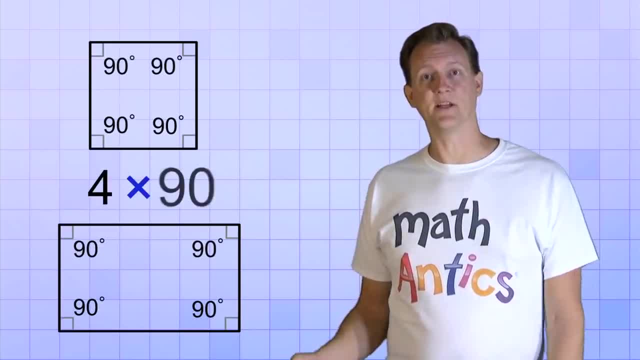 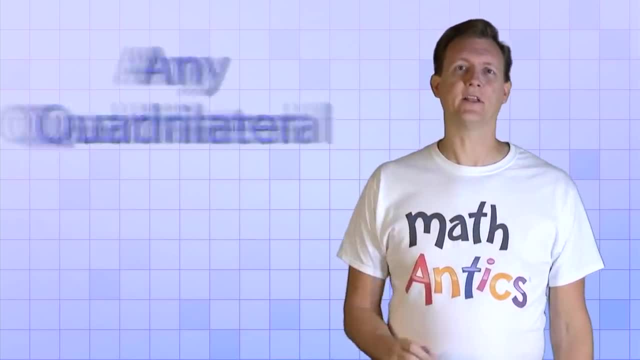 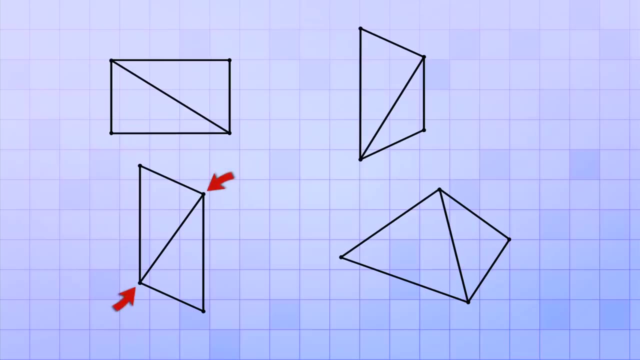 And since we know that a right angle is 90 degrees, 4 times 90 gives us 360.. But to see that it's also true for any quadrilateral, let's have a look at these four different angles. Watch what happens when we draw a line on each of them between a pair of opposite vertices. 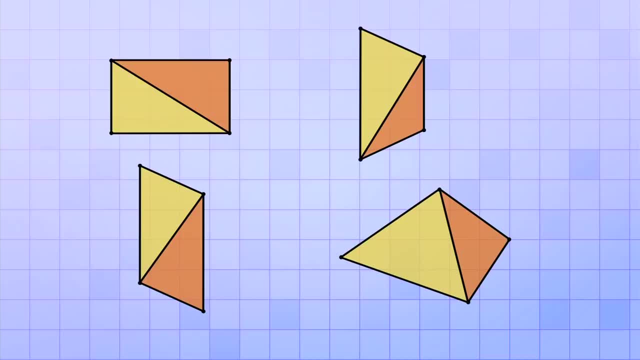 Each of the quadrilaterals got divided into two triangles. In the triangles video we learned that the sum of the angles of a triangle is always 180 degrees, So it's not too hard to see that, since the angles of a quadrilateral form two triangles. 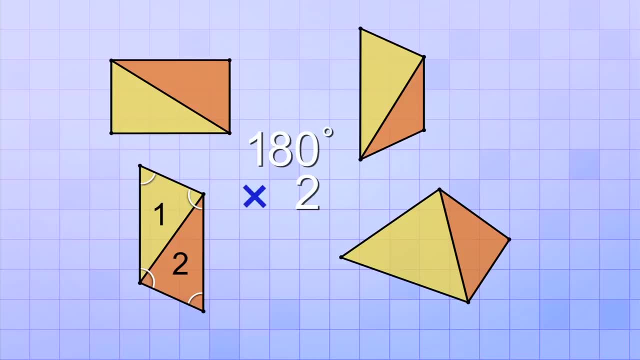 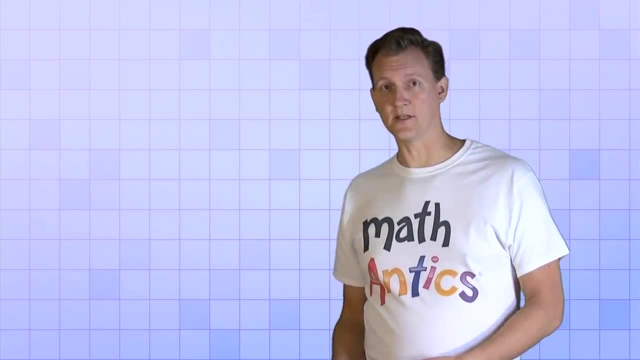 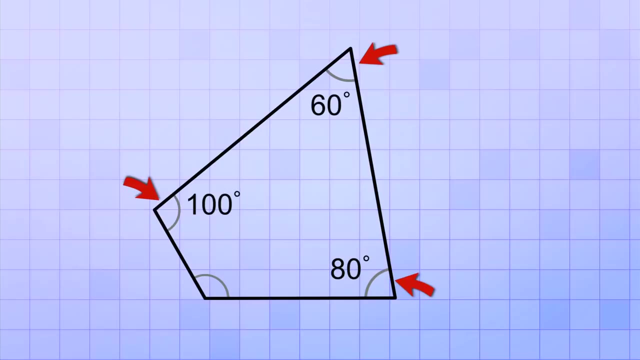 the sum of those angles would be 2 times 180 degrees, which is 360.. Knowing that the angles of a quadrilateral add up to 360 degrees can help you solve problems like this one. For this quadrilateral, we're told what three of the angles are, but the fourth one is unknown. 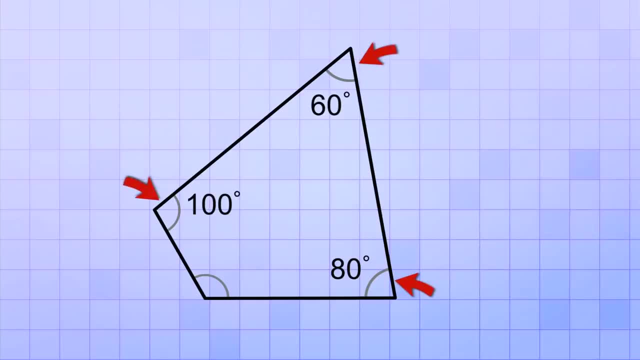 For this quadrilateral. we're told what three of the angles are, but the fourth one is unknown. To find the unknown angle, all we have to do is add up the three angles that we do know and then we subtract that from the total, which we now know is 360 degrees. 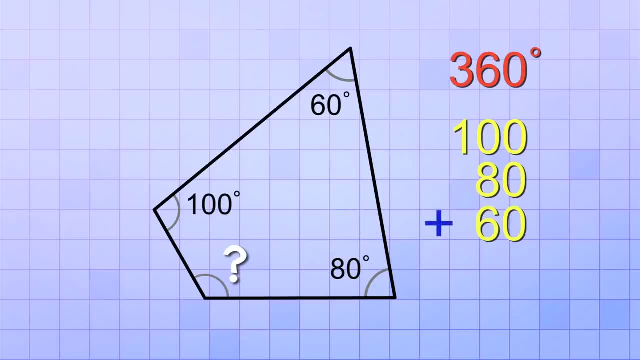 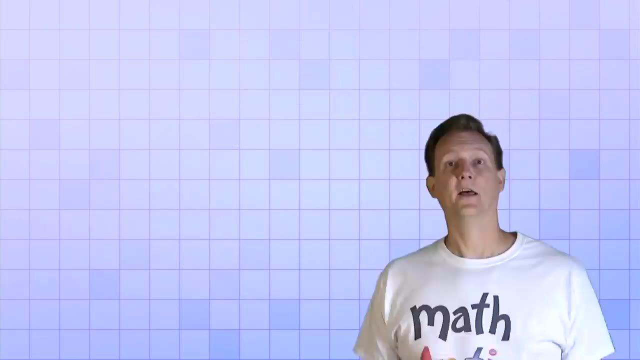 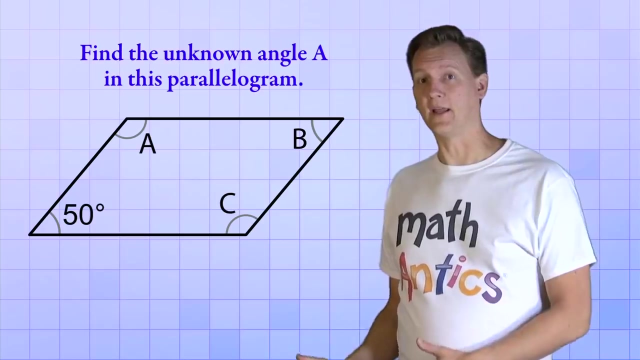 So 100 plus 80 plus 60 equals 240. And then 360 minus 240 equals 120. So the unknown angle is 120 degrees. Let's look at one more unknown angle problem. that's a little tricky. This problem asks us to find the unknown angle A in a parallelogram. 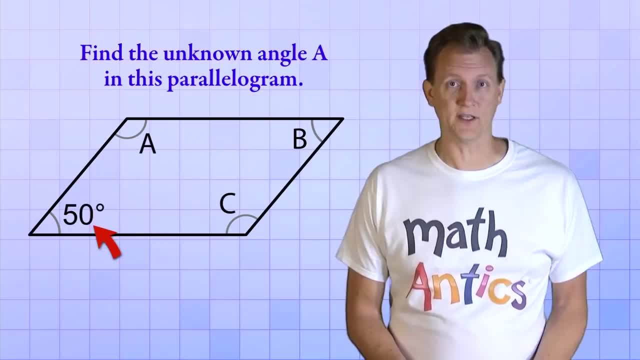 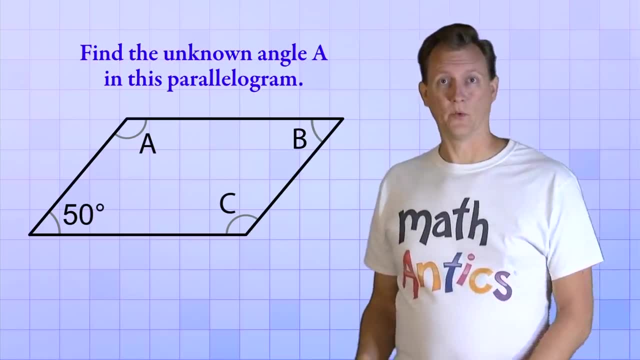 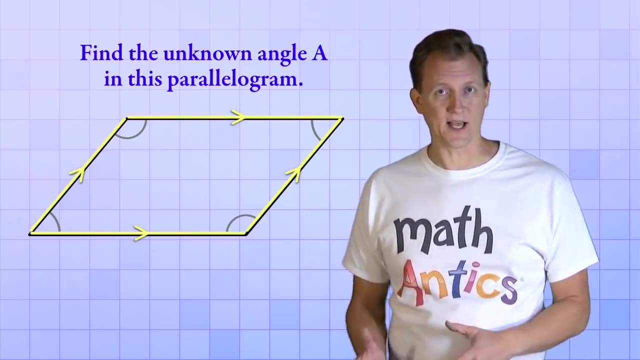 But it looks like they only told us what one of the angles is, and the other three are unknown. So how can we possibly figure this one out? To solve this problem, we need to know an important fact about parallelograms, Because parallelograms are always made from pairs of parallel sides. 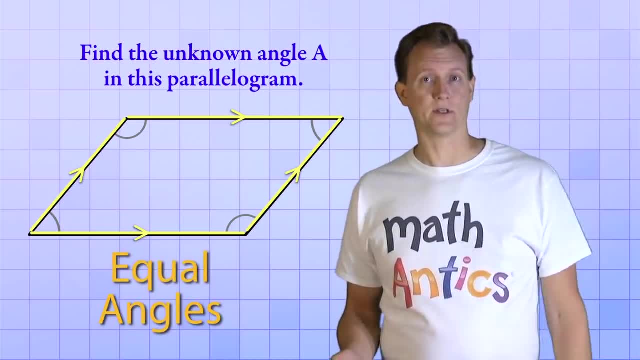 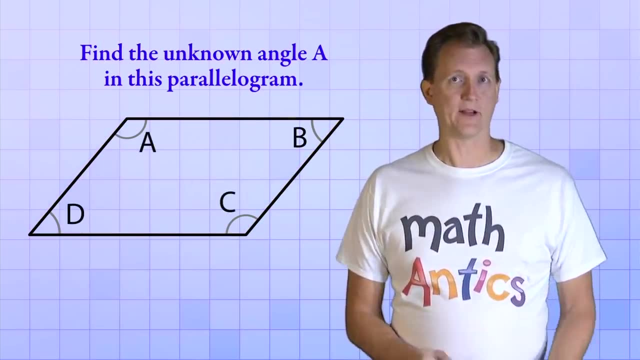 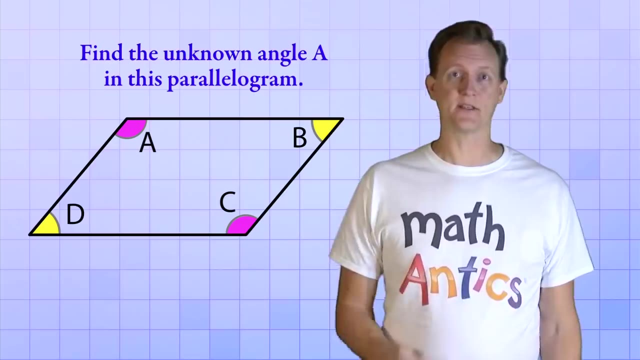 that means they also form pairs of equal angles. It's the opposite angles that form these pairs. For example, in this parallelogram, the angles A and C are equal because they're on opposite corners, and the angles B and D are equal because they're on opposite corners. 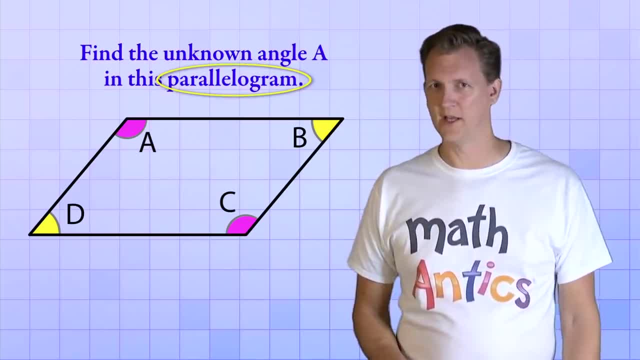 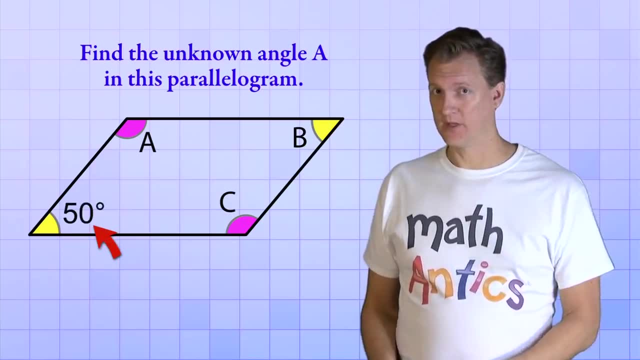 Now remember: this is only true for parallelograms. This won't work for things like trapezoids. So in our problem, even though we're only given the measure of one angle, since we know it's a parallelogram, that's all we need to figure out all the other angles. 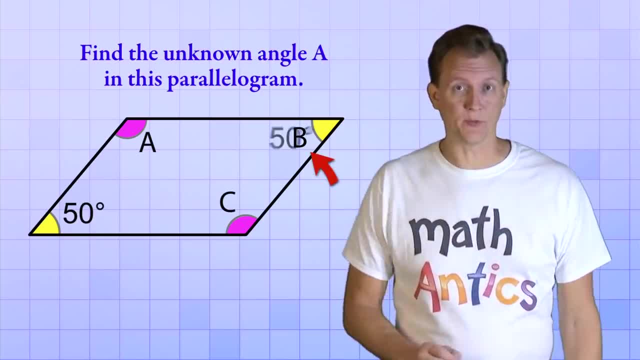 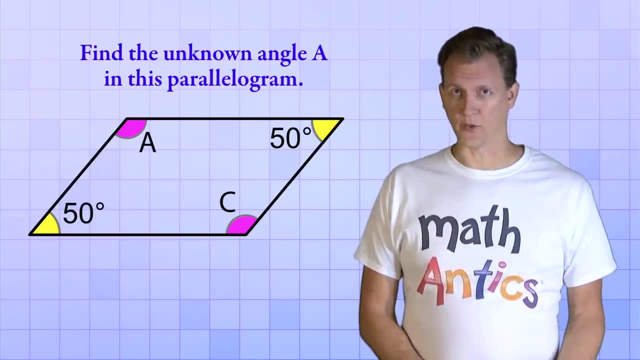 First of all, we know that angle B must also be 50 degrees, because these opposite angles must be equal. Next, we know that the other two angles, A and C, must also be equal. So if we can figure out how many degrees are left, 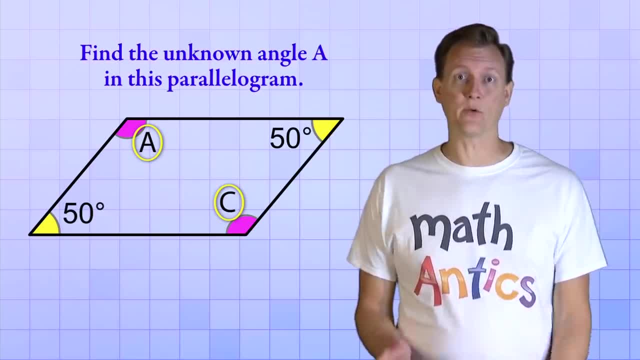 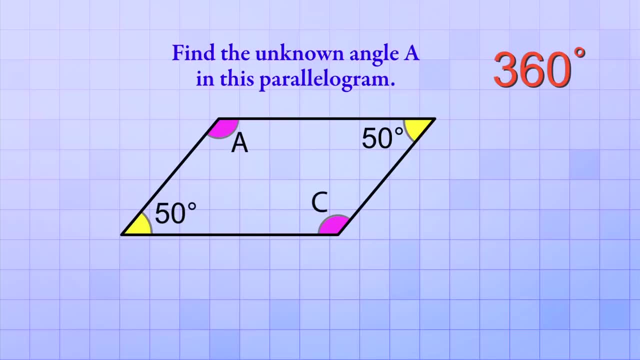 or still unknown. we can just divide that amount equally between A and C. Well, the total of all the angles is 360.. So if we subtract the angles that we know, 50 plus 50 equals 100, and 360 minus 100 equals 260,. 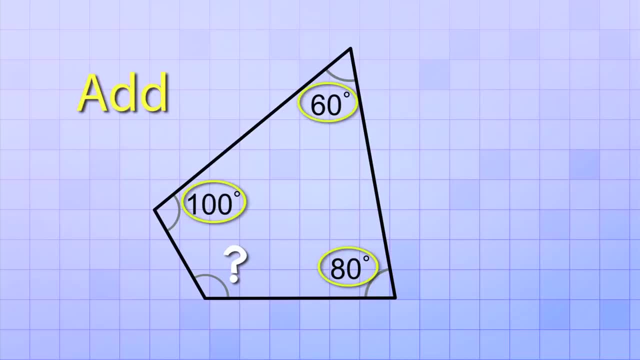 To find the unknown angle, all we have to do is add up the three angles that we do know, And then we subtract that from the total, which we now know is 360 degrees. So 100 plus 80 plus 60 equals 240.. 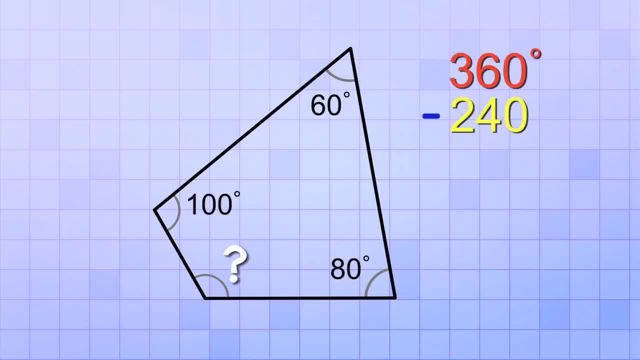 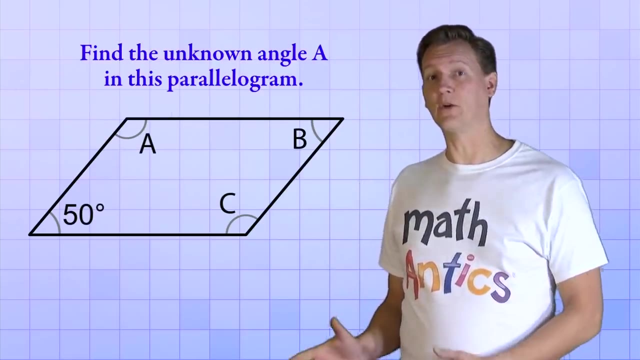 And then 360 minus 240 equals 120. So the unknown angle is 120 degrees. Let's look at one more unknown angle problem. that's a little tricky. This problem asks us to find the unknown angle A in a parallelogram. 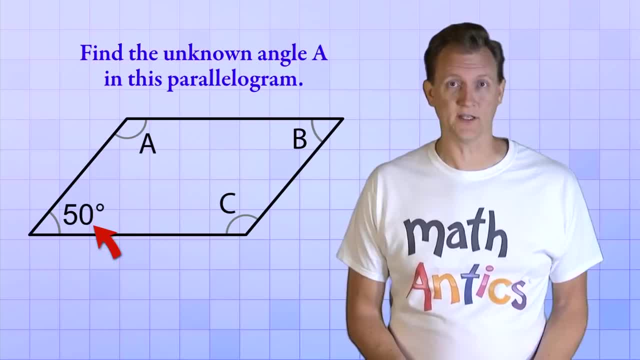 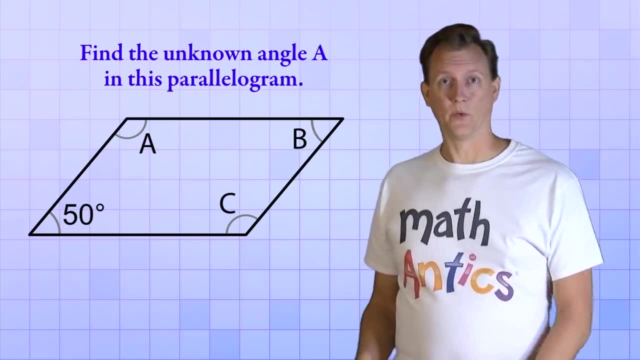 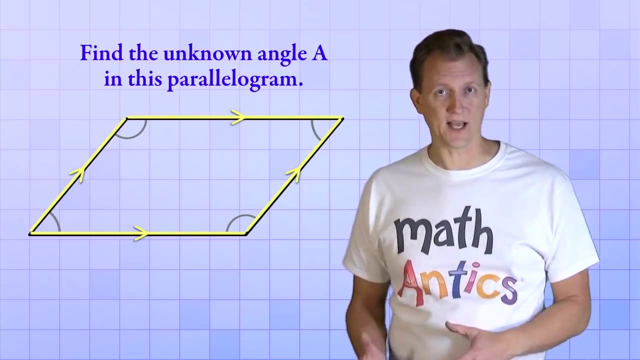 But it looks like they only told us what one of the angles is, and the other three are unknown. So how can we possibly figure this one out? To solve this problem, we need to know an important fact about parallelograms, Because parallelograms are always made from pairs of parallel sides. 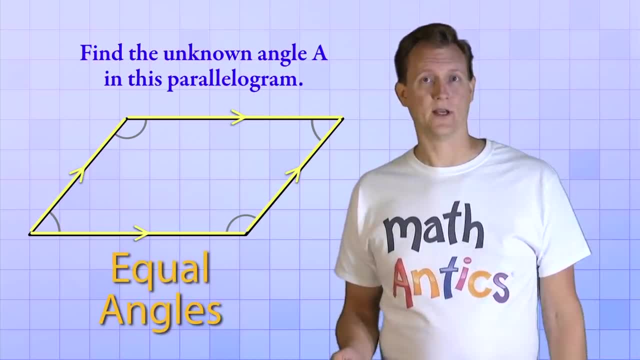 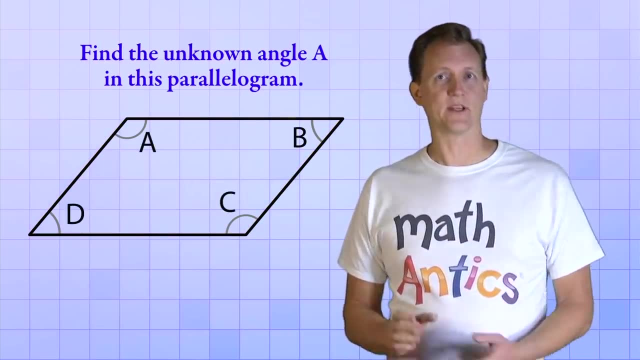 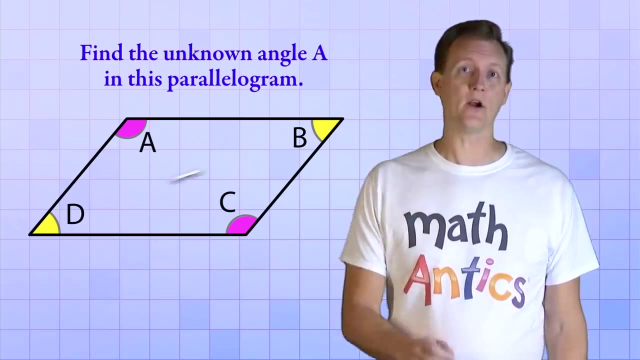 that means they also form pairs of equal angles. It's the opposite angles that form these pairs. For example, in this parallelogram, the angles A and C are equal because they're on opposite corners, And the angles B and D are equal because they're on opposite corners. 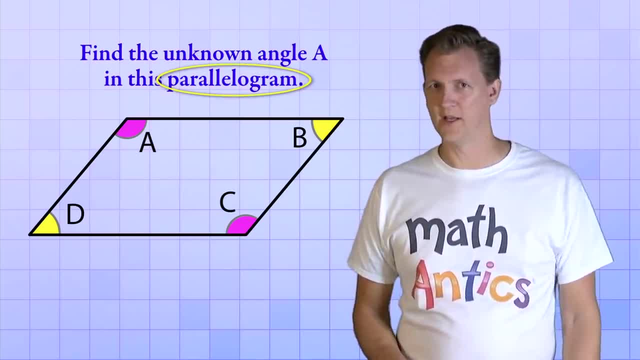 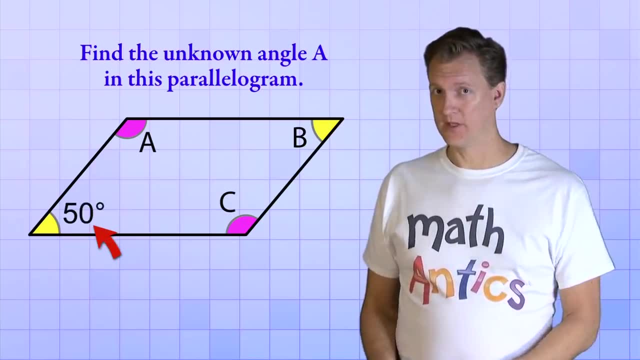 Now remember: this is only true for parallelograms. This won't work for things like trapezoids. So in our problem, even though we're only given the measure of one angle, since we know it's a parallelogram, that's all we need to figure out all the other angles. 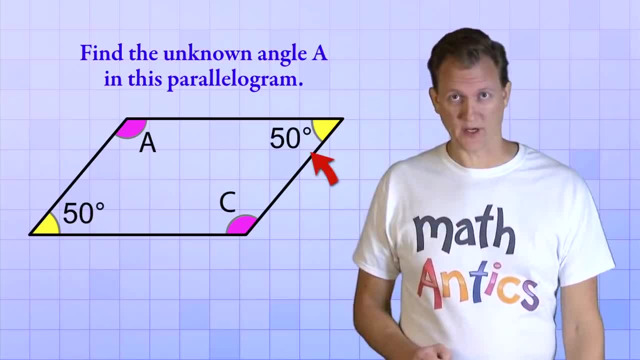 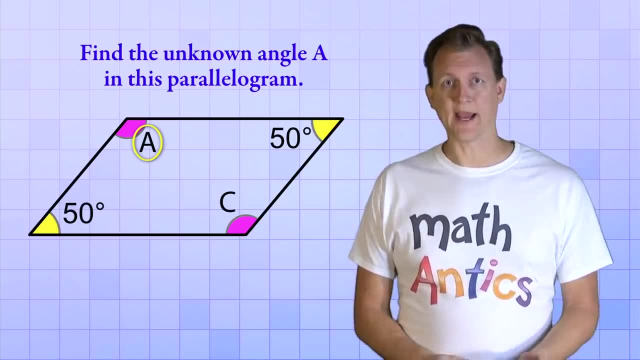 First of all, we know that angle B must also be 50 degrees, because these opposite angles must be equal. Next, we know that the other two angles, A and C, must also be equal. So if we can figure out how many degrees are left over- or still unknown- 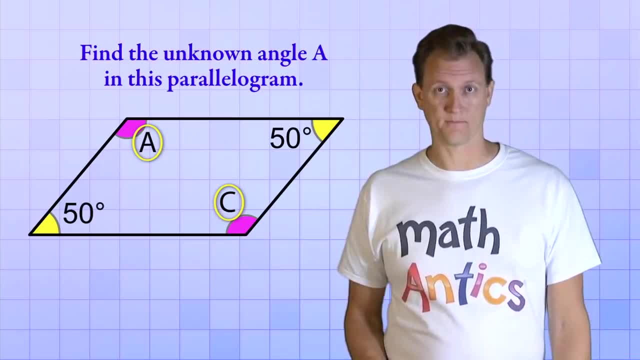 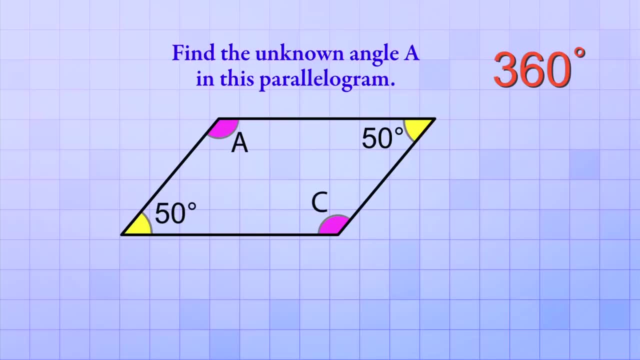 we can just divide that amount equally between A and C. Well, the total of all the angles is 360.. So if we subtract the angles that we know, 50 plus 50 equals 100, and 360 minus 100 equals 260,. 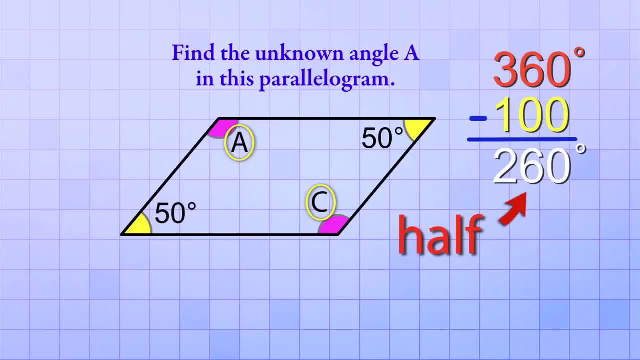 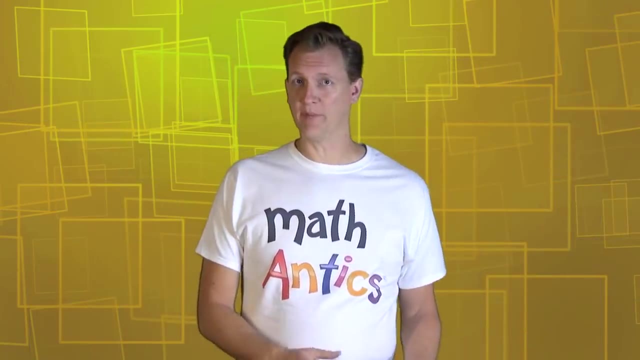 we know that A and C must each be half of 260 degrees, and 260 divided by 2 is 130, so angle A must be 130 degrees. OK, that's all for this video. We've learned the basics of how to classify quadrilaterals.